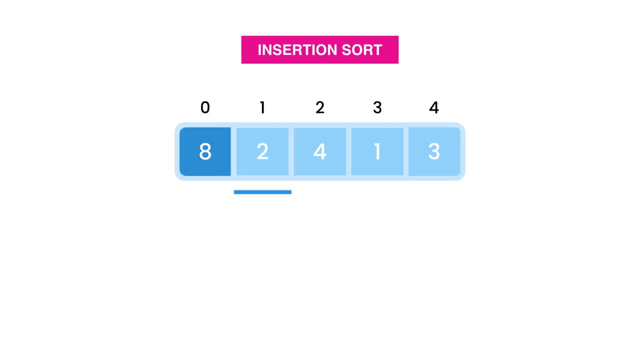 If they're greater than 2, we should shift them to the right to open space to insert 2.. This is a key distinction between insertion, sort and other algorithms we have talked about. Instead of swapping items, we shift them to the right. 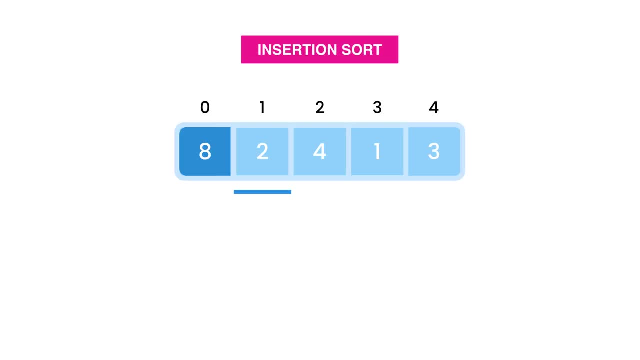 You'll see why in a second. So 8 is greater than 2, and we should shift it to the right to open space for 2.. To do this, first we store 2 in a separate variable called current. Next we shift 8 to the right. Well, more accurately, we copy it to the right. 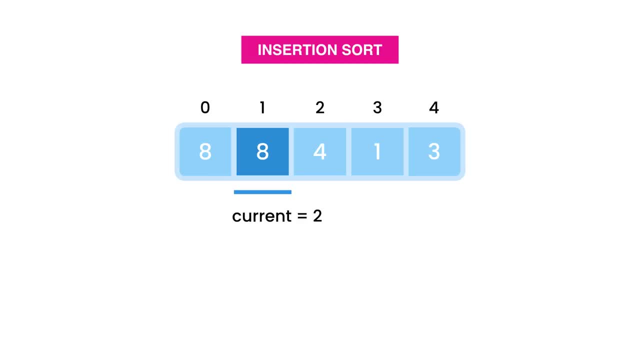 So it overwrites 2.. That's why we have to store 2 in a separate variable, so we don't lose it. Now. technically we have stored 8 in 2 places in this array, but conceptually we can assume that we shifted 8 to the right. so now, 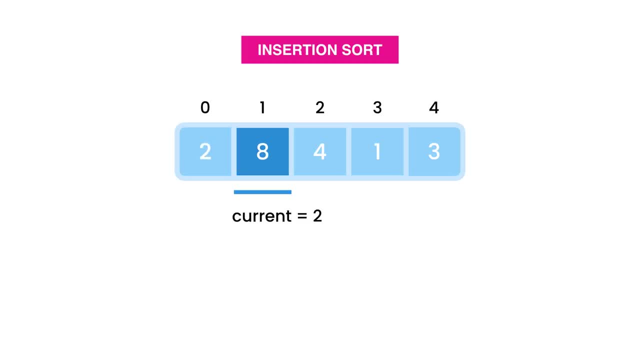 the item at index 0 is empty. So we store the value of the current variable here. So we insert a 2 in the correct position amongst the items we have seen so far. This is the sorted part of the array. In every step we pick one item from the unsorted. 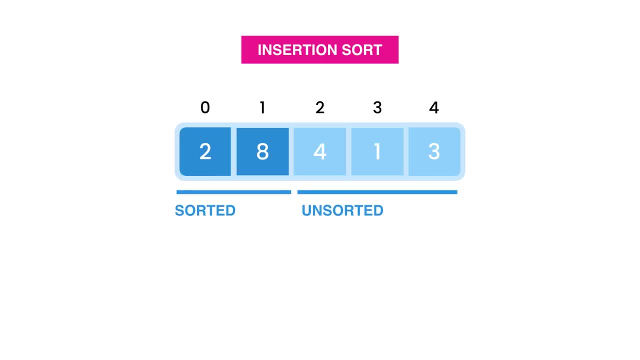 part and insert it at the correct position in the sorted part. So next we read 4.. Now we look at the items we have seen so far. If they're greater than 4, we shift them to the right to open space to insert 4.. So here we shift. 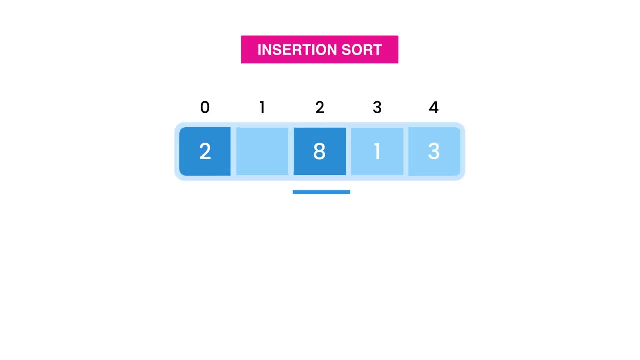 8 to the right. Now what about 2?? Should we shift it to the right? No, because 2 is smaller than 4, and it should stay where it is. So we have found the right place to insert 4.. All the items we have. 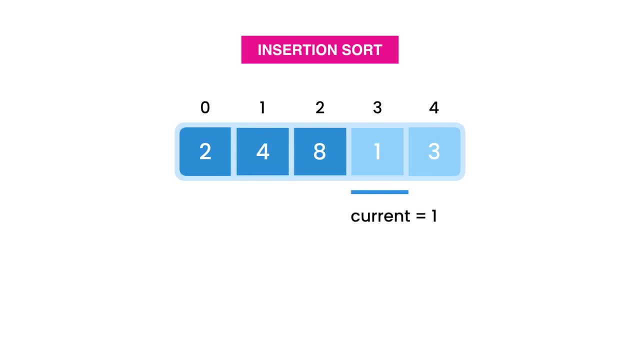 seen so far are in the correct position. So next we read: 1. Again, we should shift all the greater items to the right to open space for 1.. Here we should shift 8 to the right to insert 4.. Again, we should shift 8,, 4, and 2 to the right because they're all greater than 1.. 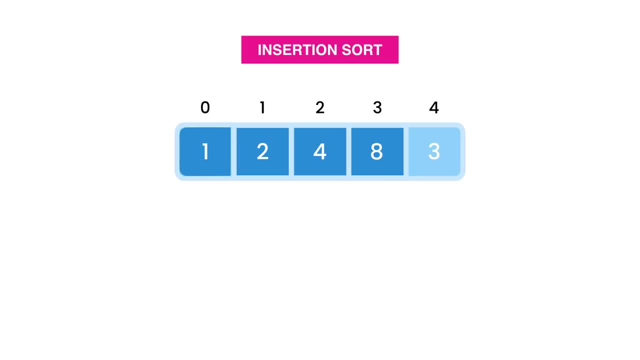 Now we insert 1 in the correct position. We're almost done. One more time We read 3 and shift all the larger items that we have seen to the right. Now we insert 3 at the correct position and we can see our array is fully sorted. So this is insertion. 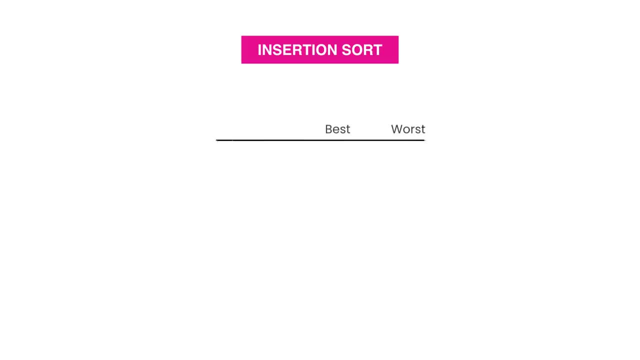 sort. Now let's do time complexity analysis. Here we need to iterate over the input array and read one item at a time. That's an O of N operation. In each step of the iteration we need to iterate over the items we have seen. 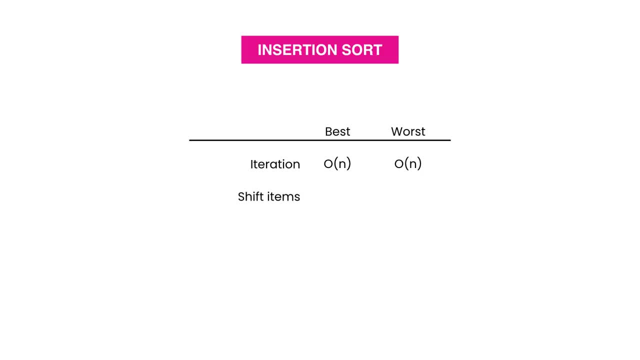 so far and shift them if required. In the best case scenario, if the array is sorted, the current item is already in the correct position, so we don't need to shift any items. That's an O of 1 operation In the worst case scenario where the array is sorted in descending order. 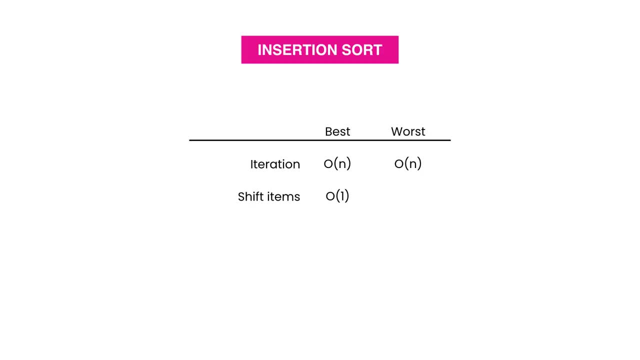 we need to shift all the items we have seen to the right because the current item is smaller than all those items. That's an O of N operation. So the time complexity analysis is now complete. The order of insertion sort is O of N for the best case scenario. 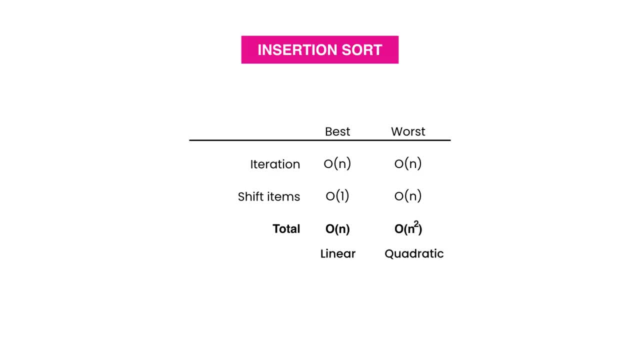 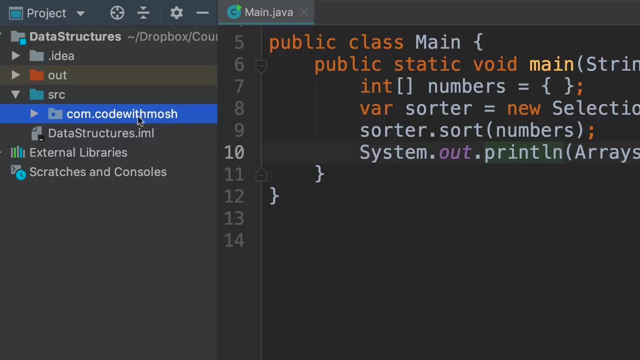 and O of N squared for the worst case scenario. It's the same as bubble sort. Now spend 20 minutes and implement this algorithm on your own. Then come back and see my solution. Just like before, let's add a new class called insertion sort. 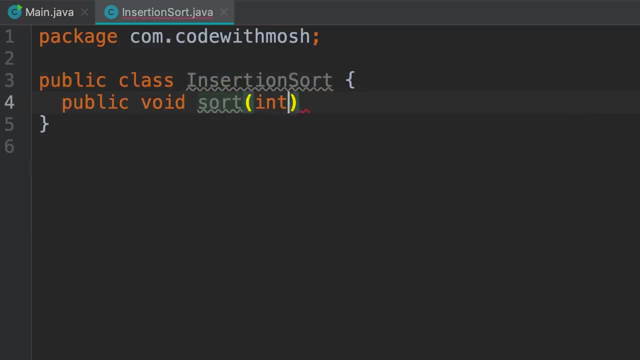 In this class we need one method, public void sort, which takes an integer array. Now here we need to iterate over this array and insert each item in the correct position. So we need a for loop. we start from index 1, because, as you saw in the previous video, 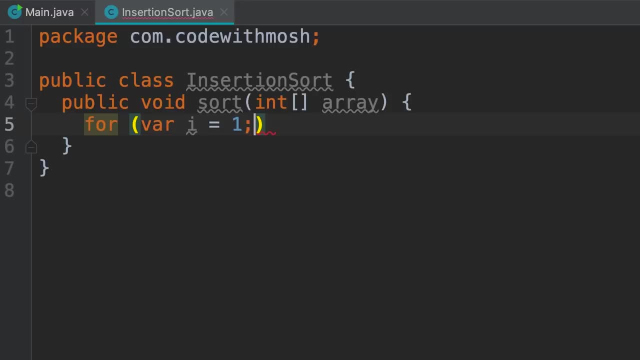 when we read the first item, we assume it's in the correct position because there are no other items that we can compare this item to. So we start at the second index. as long as i is less than arraylength, we increment i. 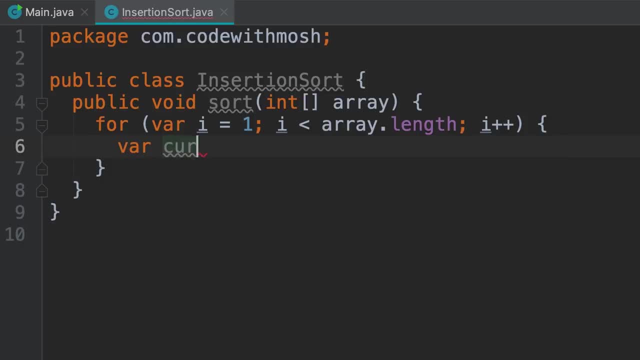 Now here we store the current item in a variable called current, So we set this to array of i. Then we need another loop to look at all the previous items, and if they're greater, we need to shift them to the right. We can use a for loop or a while loop. In my opinion, a while loop looks better here. 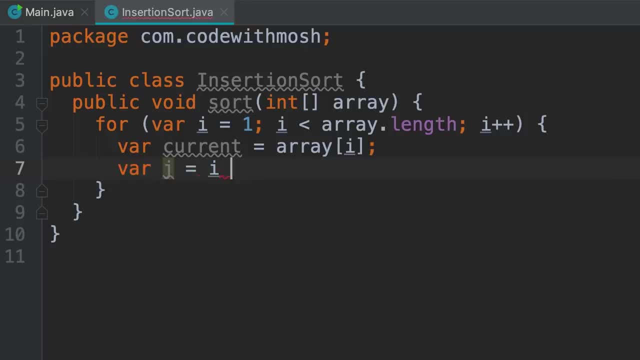 So let's say our loop variable is j, we set it to i minus 1.. We start from the previous item Now, as long as j is greater than or equal to 0, and the item that we have at this index is: 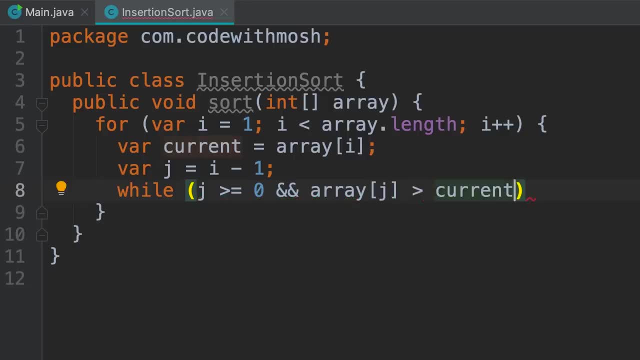 greater than the current, Then we need to shift this item to the right. So we set array of j plus 1 to array of j. So we copy the item at this index to the right side, Okay, And then we decrement j. So after this: